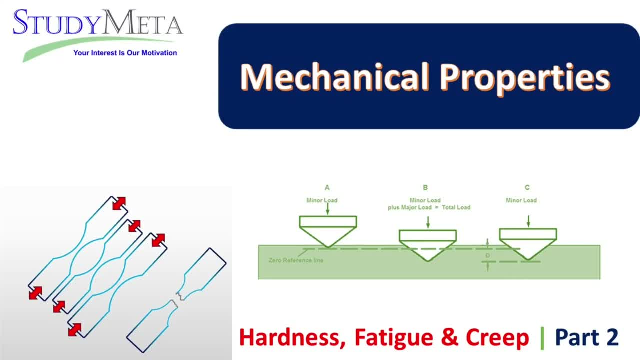 Hello everyone. today we will discuss hardness, fatigue and creep properties under the section of mechanical properties discussion. This is the part 2 of video. In previous part 1, we have already discussed the tensile properties of the materials, So let's begin with the hardness first. 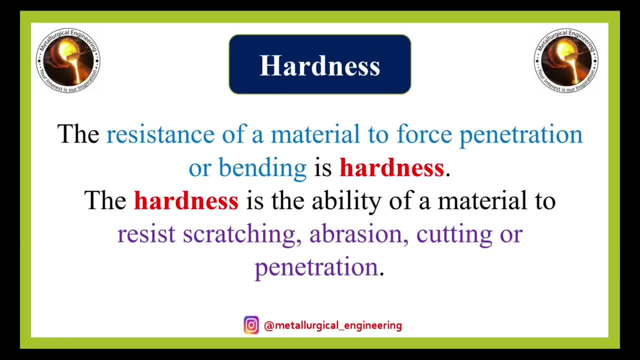 We will going to understand. another very important mechanical properties is known as hardness. Hardness is the property of a material in which the material in which it is basically, which is the resistance of a material to force, penetration or bending, bending. So it means: suppose this is your, any material and we have applied any force through this particular indenter. Suppose this is the indenter, and when it, when it. 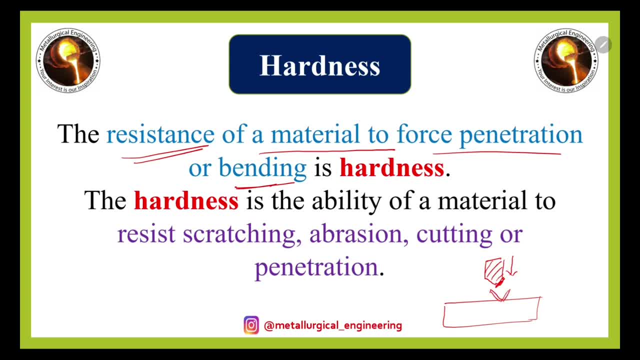 reaches up to where and it is keep moving and when it reach up to this particular metallic surface. So after this particular point it will started applying load on the material. So a material is deformed, started deforming sometime, it is deforming little bit elastically and then also and plastic reform. So it is either elastic plastic or permanent plastic or elastic also. 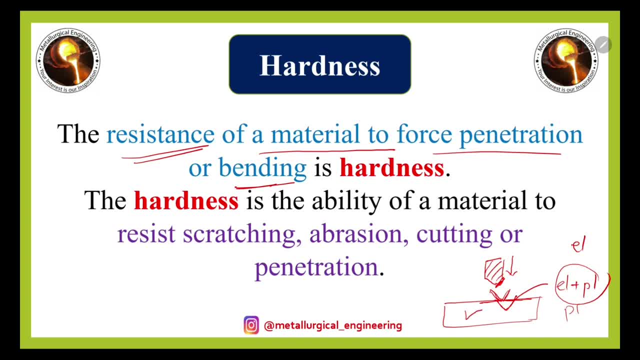 So when material is started deforming, so this material is trying to resist this deformation, Deformation. This is the Quantitatively we can. we can measure by using the hardness, or we can say: hardness is the resistance of a permanent deformation in the form of penetration or bending. 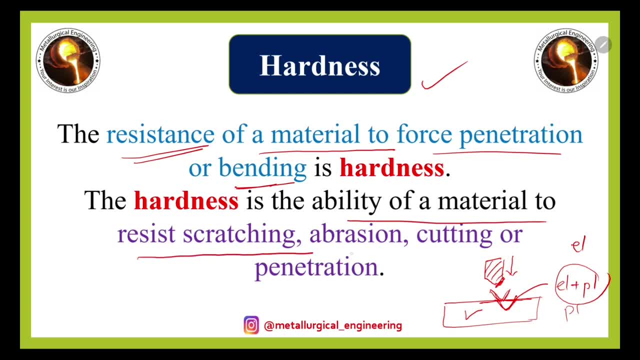 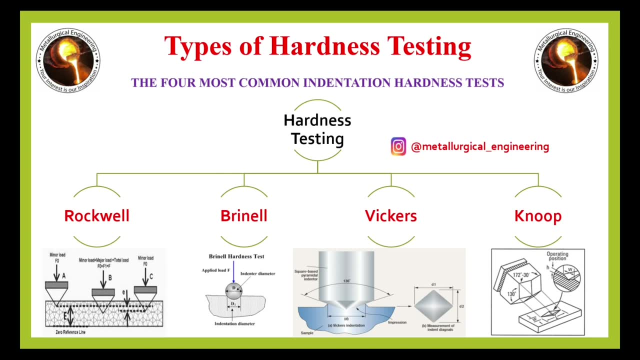 This is also the ability of material to resist scratching, Abrasion, cutting or penetration, different kinds of permanent plastic deformation. when material is resisting it is also considered as hardness Types of hardness. So hardness is basically of Basically of four types. First is Rockwell. 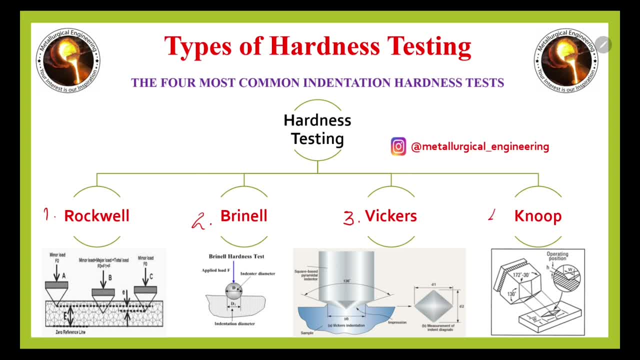 Second one is the Brenner hardness, Third one is the wicker hardness and fourth one is the loop hardness. Rockwell hardness is something where This kind of this specific type of notch is when Even is penetrating the material. So this is generally measured by the Rockwell, or this is known as the Rockwell indenter and hardness with this particular kind of 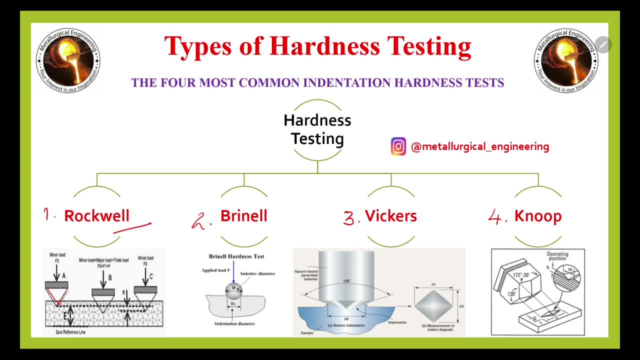 Hardness. this particular kind of indenter is known as the Rockwell hardness in Brinell hardness. basically, the indenter is a kind of a kind of solid ball, which is which is very solid compared to the material on which we are going to deform. so this kind, so with this kind of indenter, when we are 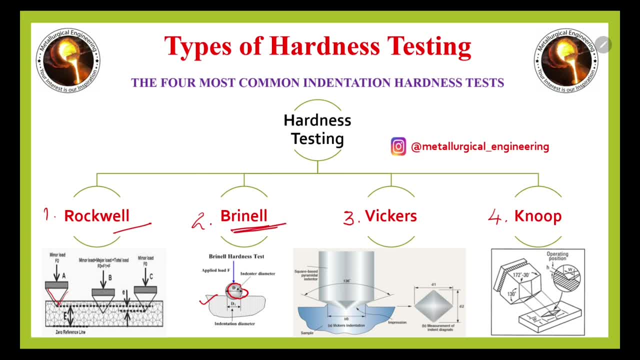 going to measure the hardness, so this is known as the Brinell hardness in wicker hardness. in wicker hardness, the indenter cross-section is something like this and an angle of this particular thing is more than 136 degree. so this kind of when indenter is going to deform the 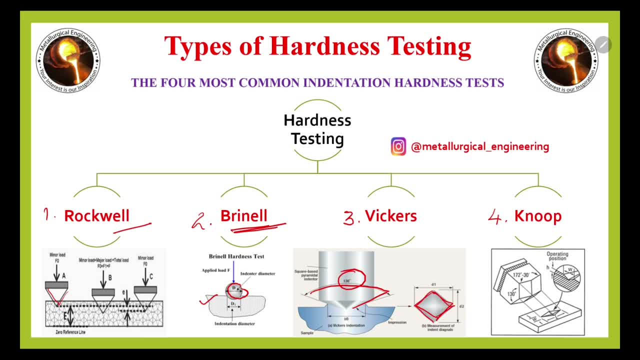 material. so this kind of impression is we can appear on the surface of the, this particular material on which we are measuring the hardness. so this is, we will measure the, its its width and its height. so this is the indenter hardness and this kind of impression is we can appear on the surface of. 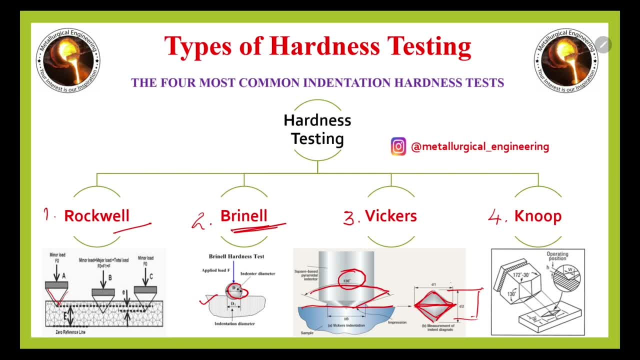 it in the form of d1 or d2 or h1 or h2, whatever we can use to measure this particular kind of indenter. so by measuring this particular point, maybe this particular parameters is known as wicker hardness. fourth, one is the noop hardness, and noop hardness indenter is something like this: 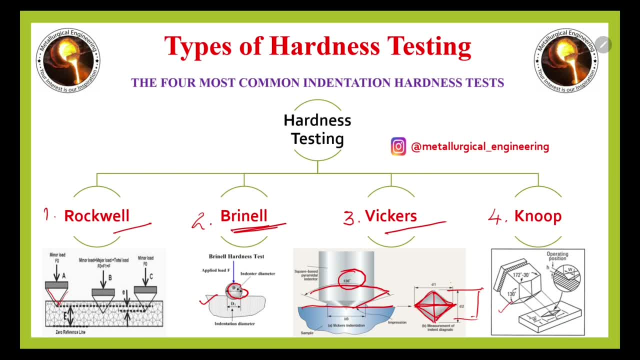 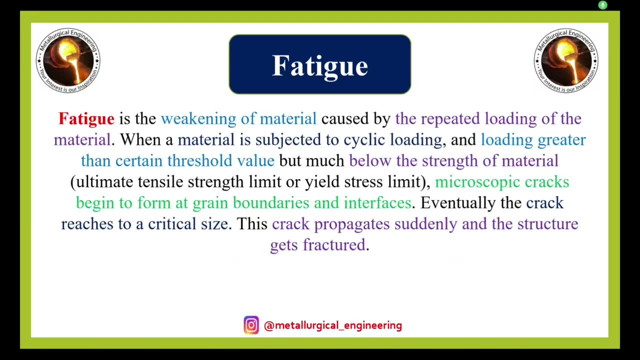 and again the material is going to deform again. this, in this kind of indentation, is known as the noop hardness. now we are going to understand several very important time varying mechanical properties, phenomena, and one of that kind of property is known as the fatigue property. fatigue, the term itself itself is, is, is is showing the definition, showing its definition. 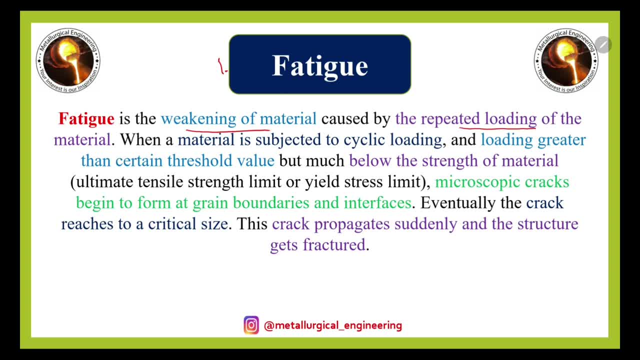 where material is going to slowly weaken under the repeated loading, under the repeated kind repeated loading. so here we can. a very important thing is the weakening of material, and under the repeated loading it means. suppose we have any specimen and we apply any load repeated loading, so material is slowly going to, slowly going to weaken. with how much? 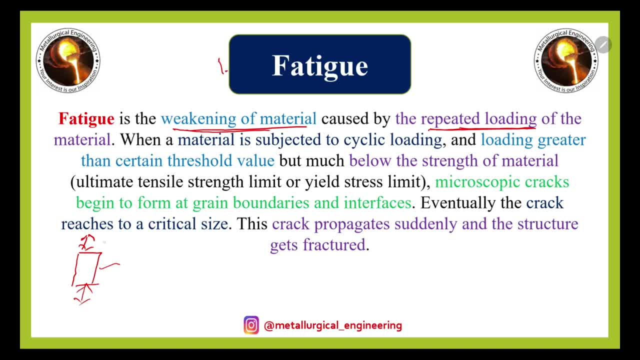 number of repeated loading is applied. this repeat number of repeated loading is something count in terms of number of cycle of that particular loading. so with that number, how much number of cycle is performed to weaken this material? is known as the fatigue. fatigue means material is going to weaken and some other very important terms associated to the fatigue and those terms. 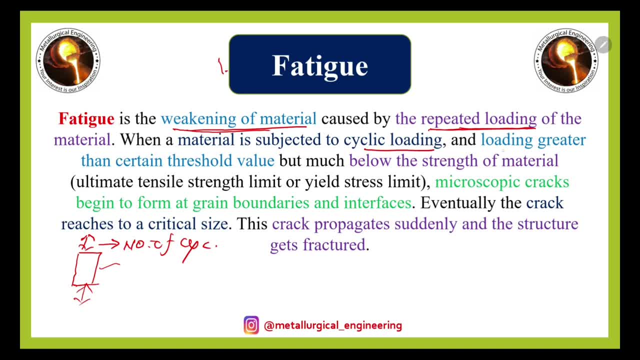 are like cyclic loading, which is applying greater than the certain threshold value but much below the strength of the material. so this strength of the material, as we already explained in tensile property, that is ultimate tensile strength limit, ultimate tensile strength or yield stress, so the limit of this, 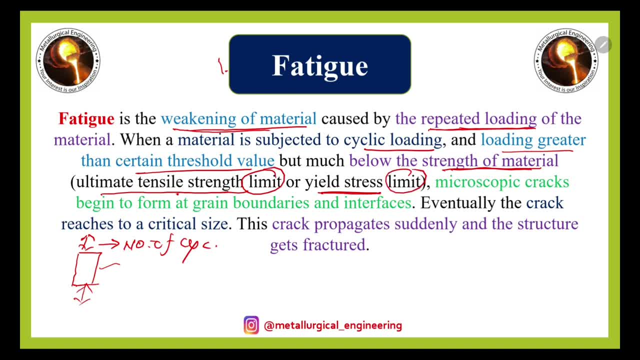 particular tensile strength or yield stress, our applied repeated loading, the maximum applied, the maximum, the maximum load of the maximum load of this repeated loading should be lesser than this. this kind of limits, whether it is ultimate tensile strength or yield strength, but it is certain, above to the threshold value, or suppose the yield strength of the material is. 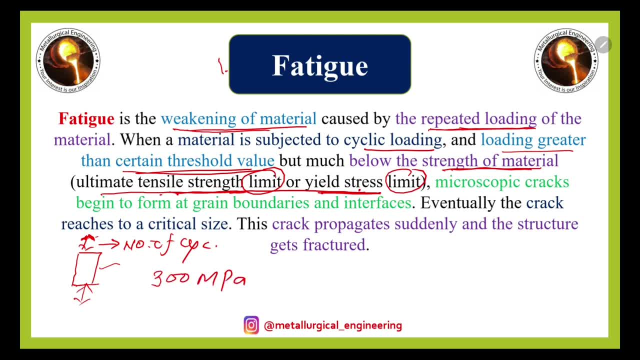 like 300 megapascal. so we have to apply the repeated loading which has two- uh two- load conditions: one is maximum applied load or maximum stress, and another, another is the minimum stress. so this maximum stress should not cross this um tensile strength of the material and the Sigma minimum means a minimum threshold value of between 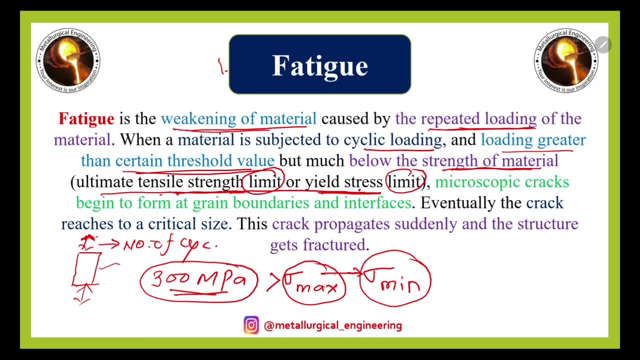 these, between these two minimum and maximum loading, we apply the load in cyclic, cyclic form, so this is known as the cyclic loading. so with this cyclic loading, when we apply, material is slowly started weakening and at particular point it's going to be fracture. so the fracture now. now the third term is: 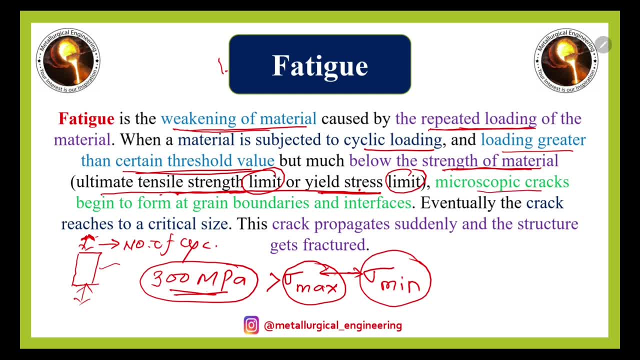 appears fracture. so fracture is something which is, uh, macroscopic crack. it's this fracture is basically happens, but before happening the fracture that those cracks suppose, this is the material and when we apply the cyclic loading on this particular material. so initially any micro crack appears on the material surface or interior of the material. mostly these cracks or microscopic 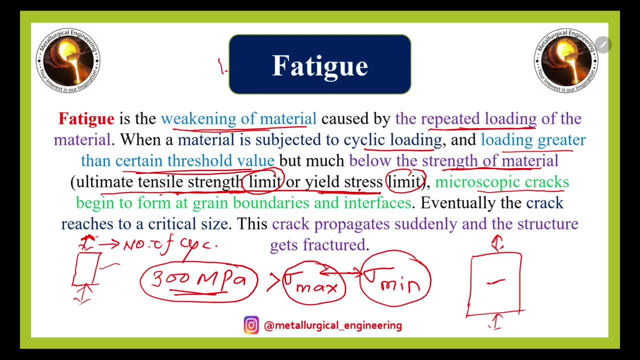 cracks, which is very initial stress of the fracture. it appears generally on this surface of the. this material surface means suppose, this is the surface, so from here, this is the surface of front, front, front of the, this particular specimen. so this crack started appearing from the surface and with, with